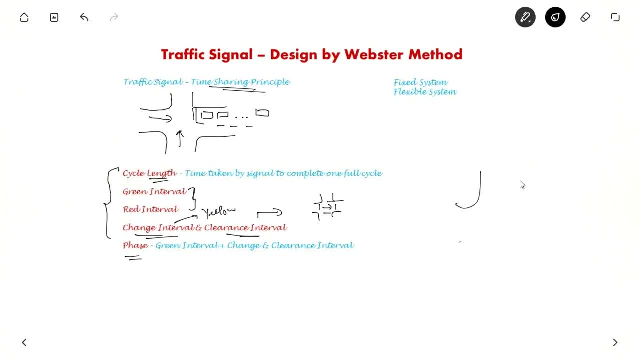 What is a phase? So first, if suppose this side goes, all three directions are possible. So this is one phase. The second phase is like this: So there are four phases in a four armed intersection. So that is a phase. One phase is green interval plus change and clearance interval. 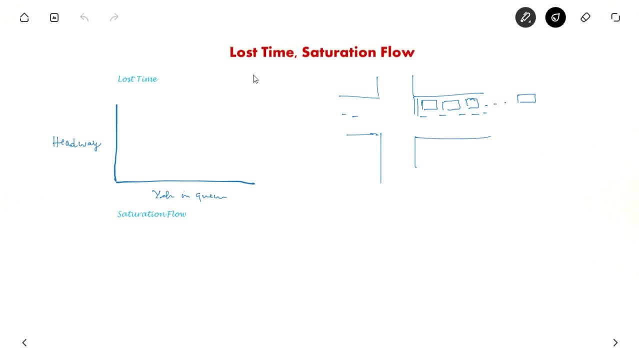 Before we move on to Webster design, there are two important terms which you need to know. One is loss time and another is saturation flow. Suppose this is the first vehicle, second vehicle, third vehicle and this is the nth vehicle waiting during red time. Now this side becomes green, So the first vehicle takes some seconds to start. 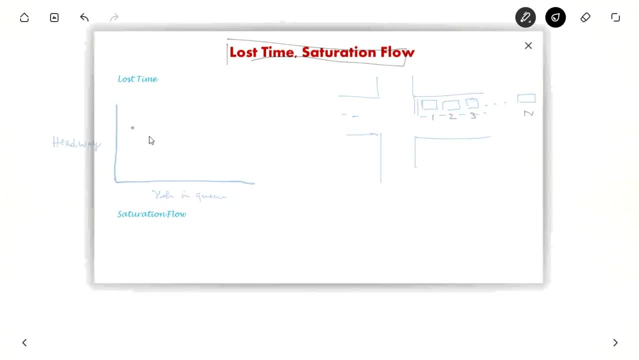 And the second vehicle takes lesser amount to start, because for the first vehicle It takes some time to react that the signal is green and then only it starts. So the second vehicle takes little lesser time And the third vehicle takes even lesser time. 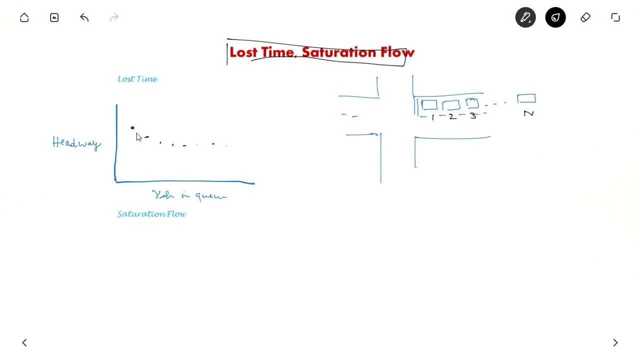 After one particular time it becomes Constant. So this constant time is the headway, So it is constant headway, and so the extra time taken by the first few vehicles is called the lost time L, So there will be a lost time for each phase. 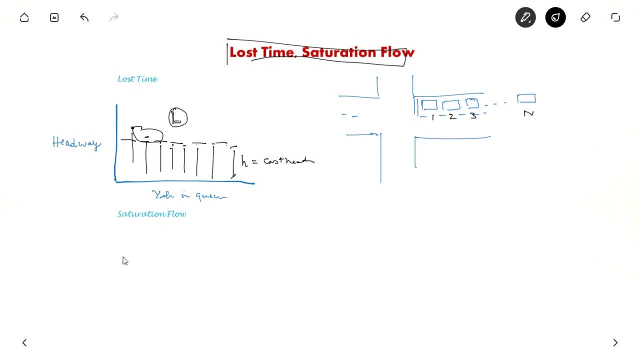 Saturation flow is nothing but the highest amount of flow possible. So saturation flow is inverse of headway. This constant headway which we see, that is saturation flow. Saturation flow equal to 1 by headway, If headway is in seconds and you need saturation flow in vehicles per hour, so it is 3600 by 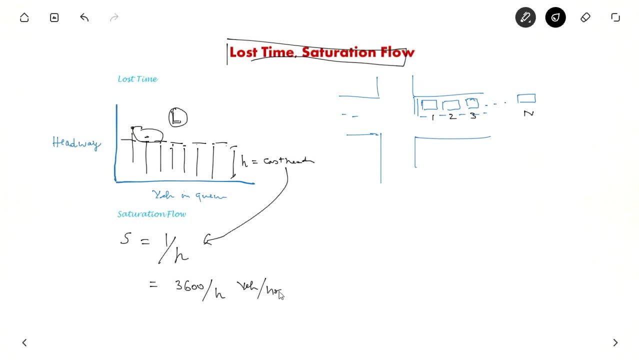 h vehicle per hour. So this is saturation flow. Here I will explain how the signal works. Suppose this is the start of red time and here this is the number of vehicles. number of vehicles. So if suppose red time is for 30 seconds. 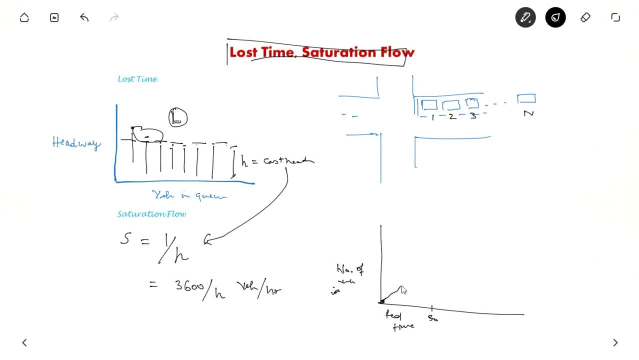 So vehicles start keep on queuing. First, 5 vehicles arrive, 10 vehicles arrive, 20 vehicles arrive, like that. After that it is green time, So the vehicles keep on queuing, So the queue reduces. So this is discharge of vehicles during green time. 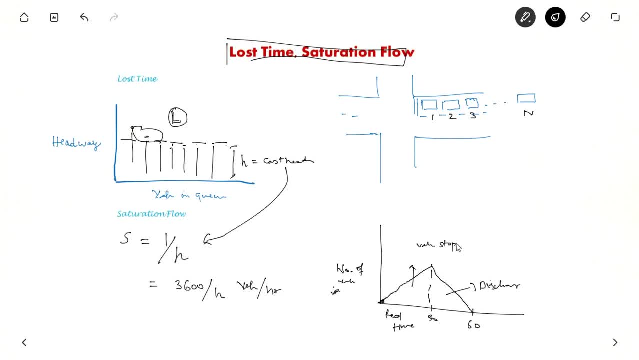 And this is vehicles stopped in red time. So this area will give you the delay during red time. Now we will move on to the Webster method. So these are the important terms associated with Webster method. First, what is saturation flow? you know, and observed volume is saw volume, observed in. 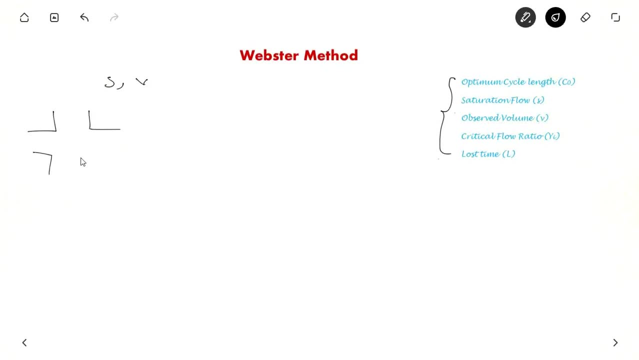 each phase. Here saturation flow for this phase will be 1 by h and volume is the volume which you observe on the road. So this is saturation, So all these segurança conditions we know. So saturation flow in case of refraction road, So critical flow ratio- this is a very important term: critical flow ratio y, i, y. 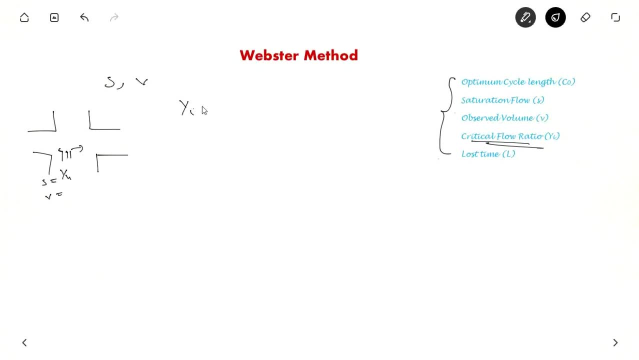 i represent each phase, So there are four phases here. So y i equal to v i divided by s i, So it is nothing but volume by saturation flow. This ratio is called critical flow ratio. So for four phases there will be four critical ratios: y 1, y 2, y 3 and y 4.. Like y 2 is 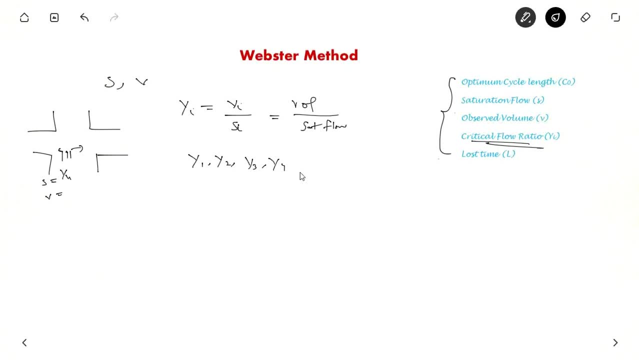 v 2 by s 2, y 3 is v 3 by s 3 and so on. And what is loss time Loss time. as you saw, because of some vehicle discharge, first few vehicles took lot of time. So that is why.